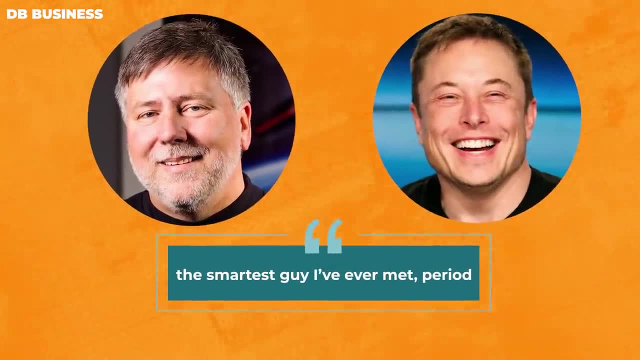 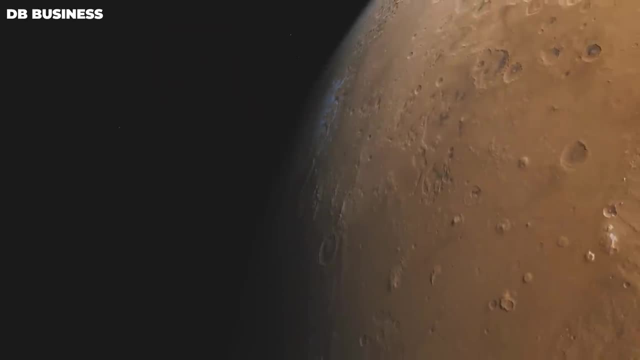 Musk would later describe him as the smartest guy I've ever met. period Musk told him over the phone that the two of them needed to speak, and he eventually probed Cantrell for information about the possibility of sending a spacecraft to Mars. The future SpaceX founder had just been rejected. 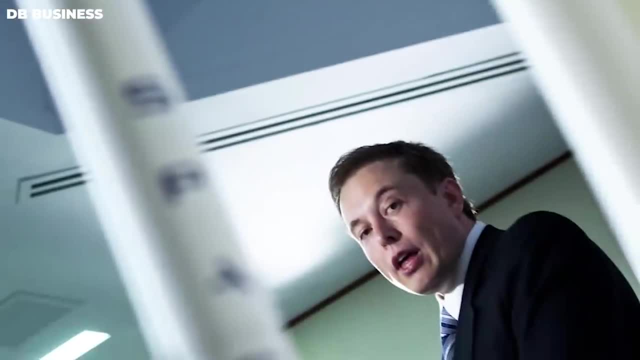 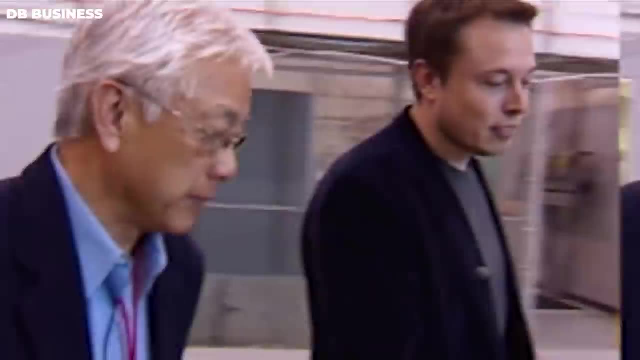 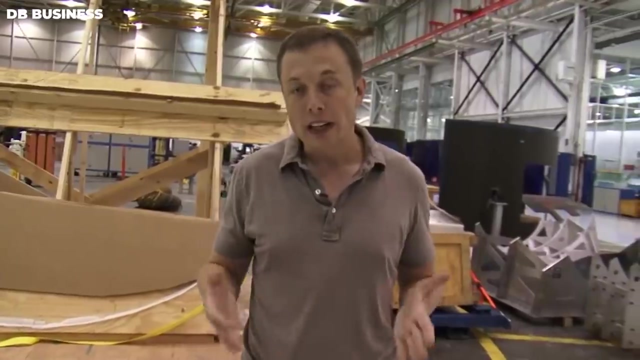 by the Russians and was looking for a little guidance. Allegedly, Musk had gone to the Mars, but the price tag was enormous At the time. Musk was not a billionaire, though had made a few millions, so he could not afford what they were asking. His solution: Build the rockets himself. 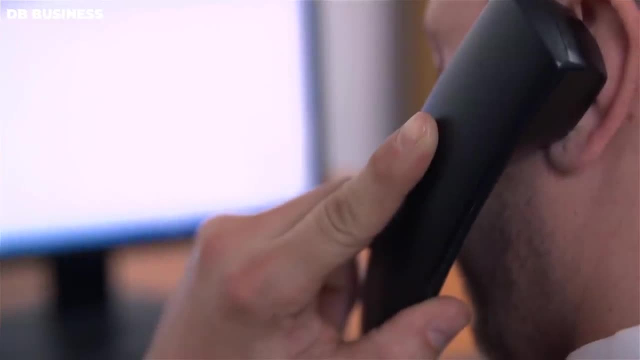 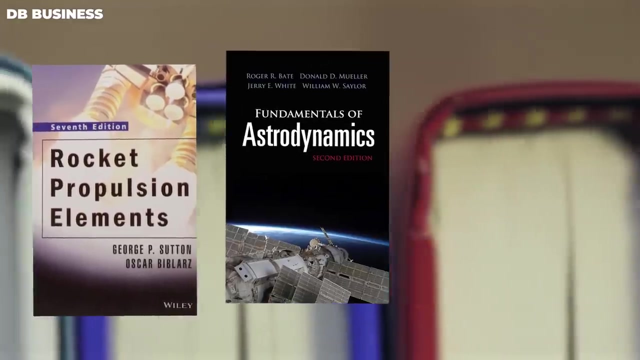 That's where Cantrell came in. Cantrell, intrigued by the proposition, allowed Musk to borrow some of his textbooks. He lent him titles such as Rocket Propulsion Elements, Fundamentals of Astrodynamics and the International Reference Guide to Space Launch Systems, just to name a few. Musk poured. 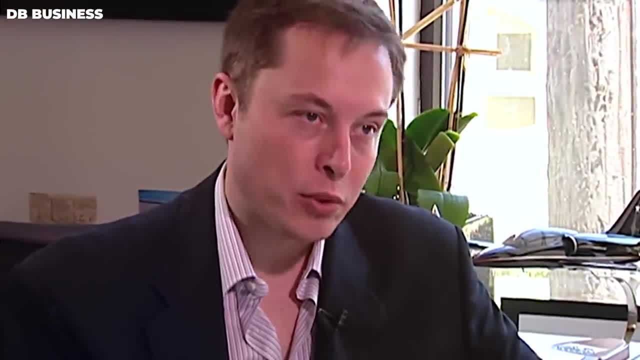 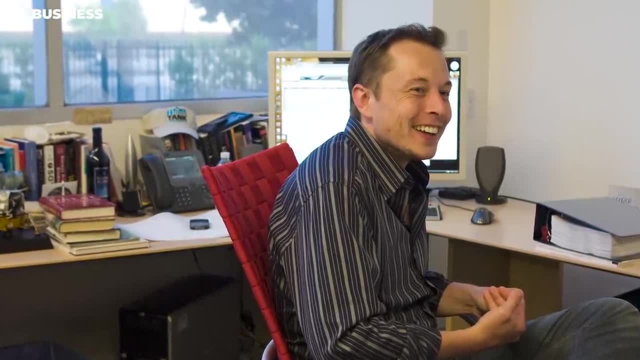 over these titles and he was able to do what he wanted to do. He was able to do what he wanted to do. Cantrell would later say that he was unsure whether or not Musk took notes on the information in the books, but what he does know is that Musk appeared to have memorized close to everything. he 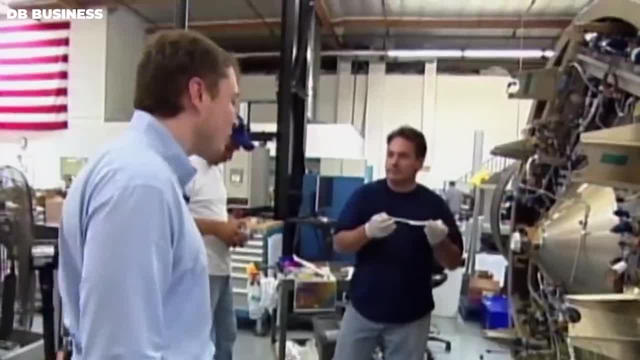 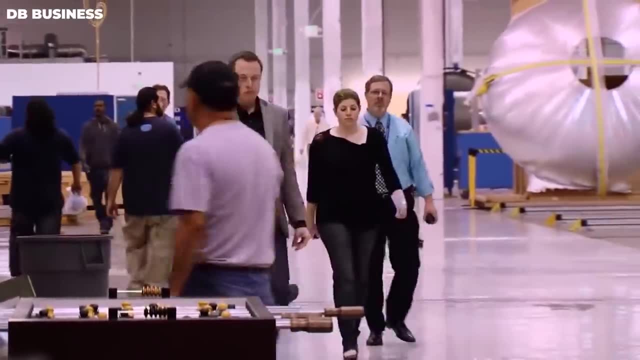 read. Because of this, Musk was equipped with the knowledge and the vocabulary to carry on conversations about rocket science, astrodynamics and other topics. After reading the textbooks, Musk developed the very plans for the rocket that would eventually be used by SpaceX. 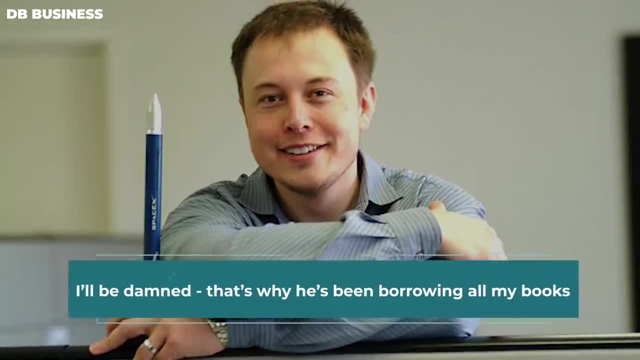 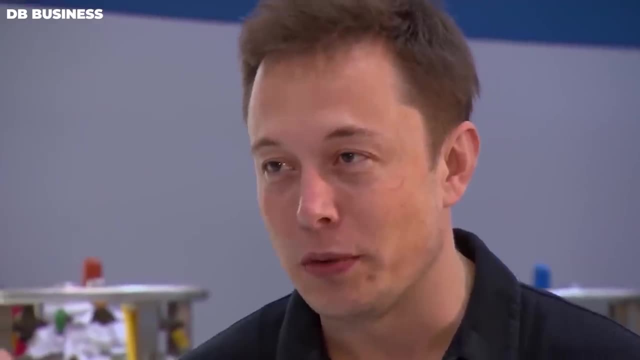 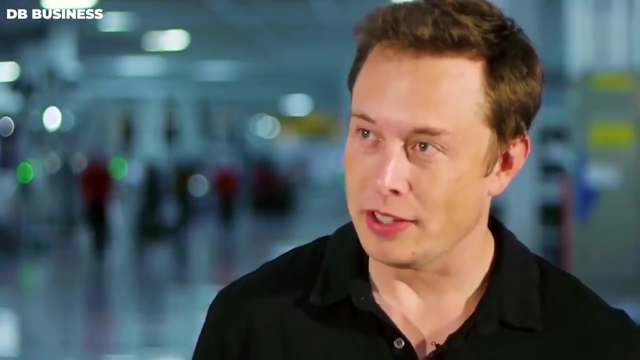 Cantrell recalls thinking to himself: That's why he's been borrowing all my books. The mechanical engineer was impressed not only by how much information Musk had absorbed, but how much he had applied In addition to collecting textbooks. another principle that Musk follows in his quest for self-education is surrounding 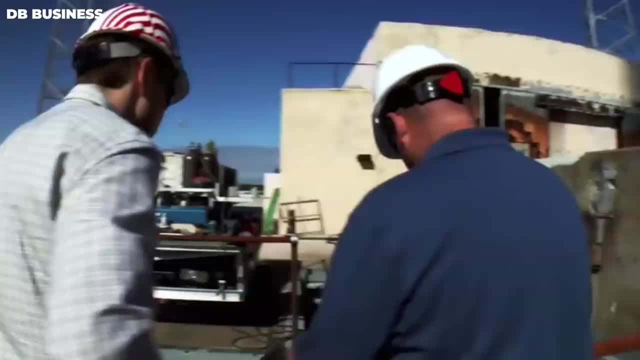 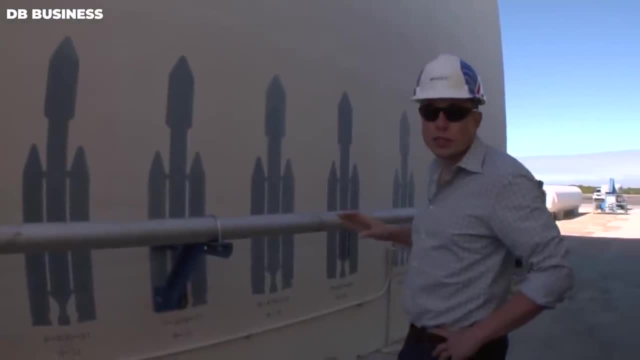 himself with the best and the brightest. He would strike up conversations with people who were the best in their field, acquire their knowledge and expertise through discussions and then try to replicate that knowledge when he applied it to his endeavors, Such as with space and space and the. 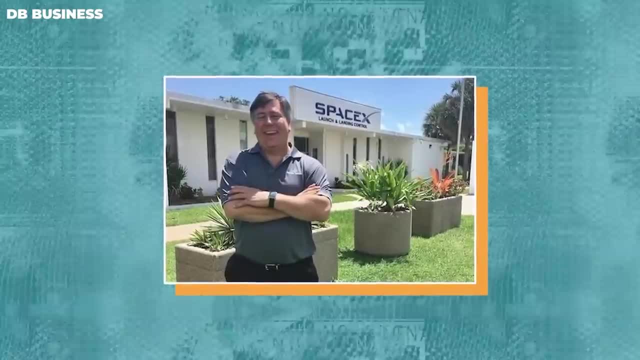 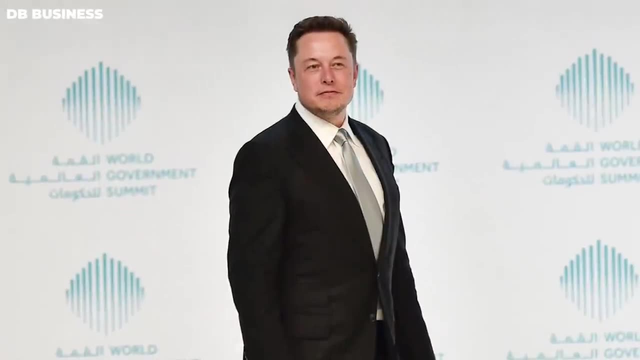 best in their field. In fact, Jim Cantrell actually worked with Musk at SpaceX for a time before moving on to his own ventures. Speaking in Dubai at the World Government Summit in 2017, Musk said this about the power of asking the right questions. 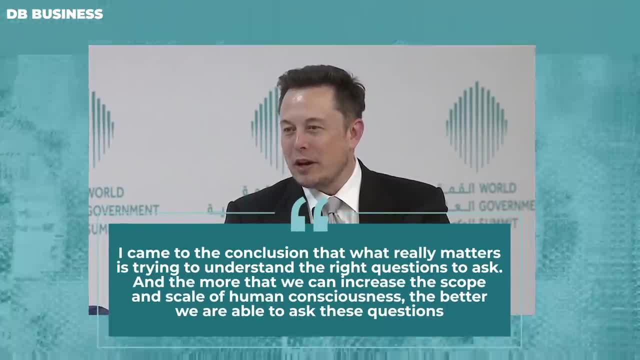 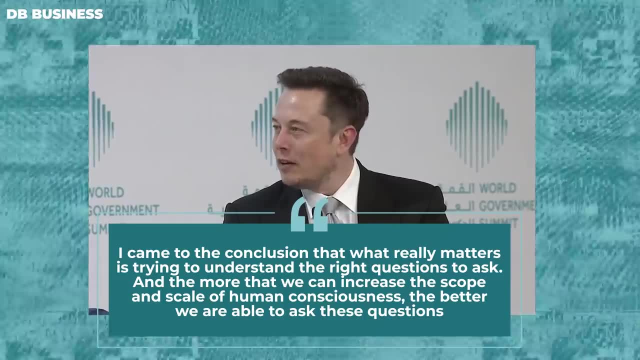 I came to the conclusion that what really matters is trying to understand the right questions to ask, And the more that we can increase the scope and scale of human consciousness, the better we are able to ask these questions. It is for this reason that he keeps. 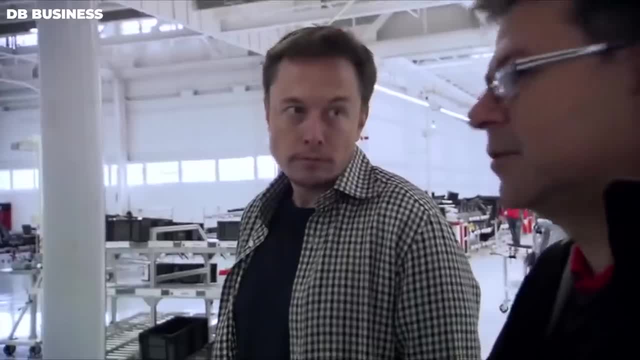 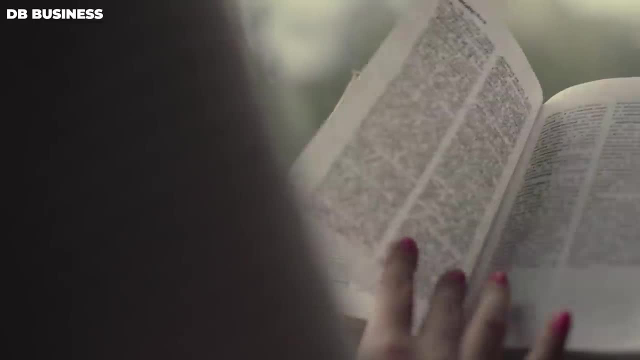 a close network of industry experts, some of whom he even employs. You might be asking: just how much reading does it take for someone to become a self-educated rocket scientist? The answer is quite a lot. In a 2017 interview with Rolling Stone, Musk admitted that he was. 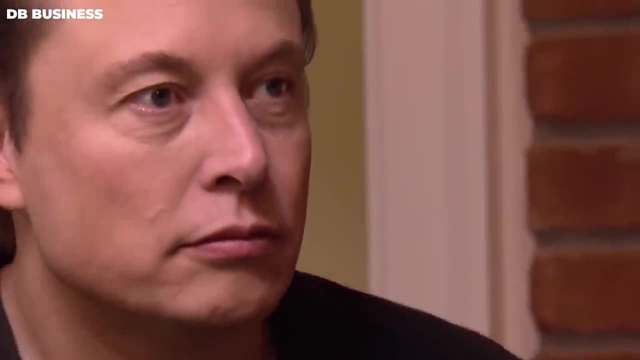 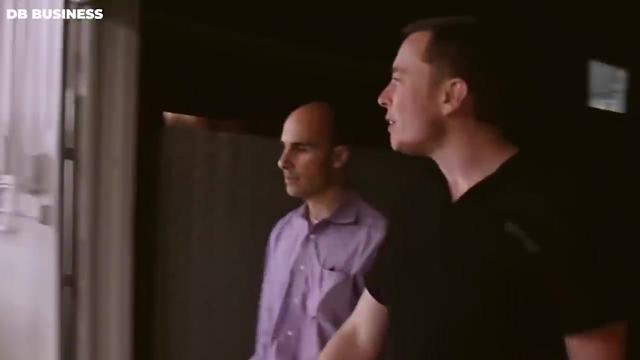 raised by books and then my parents. He credits his time spent reading to how he became as successful as he is today, and his reading history is an impressive one, as you might have imagined. The famous adage of all trades is a master of none is definitely not applicable to Elon. 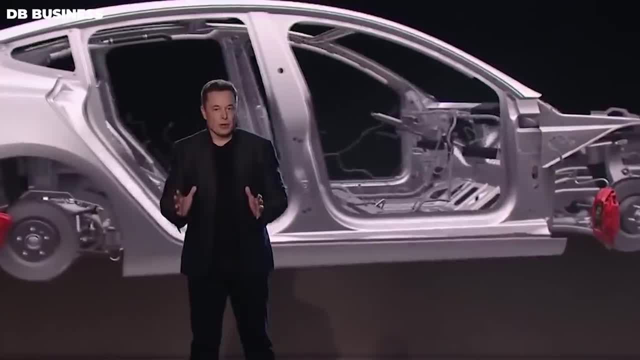 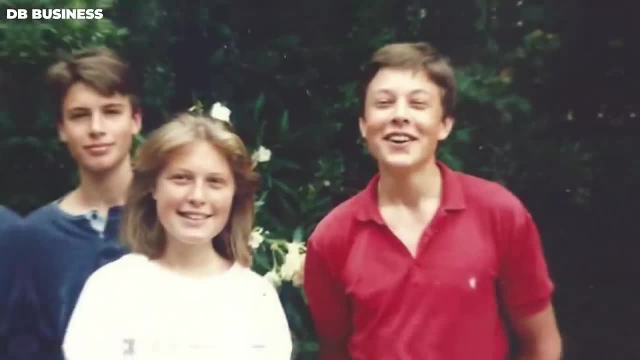 because he is a great example of someone who is very successful across multiple areas. When he was just nine years old, he reportedly read the entire Encyclopedia Britannica, then moved on to almost exclusively reading science fiction novels for about 10 hours per day. 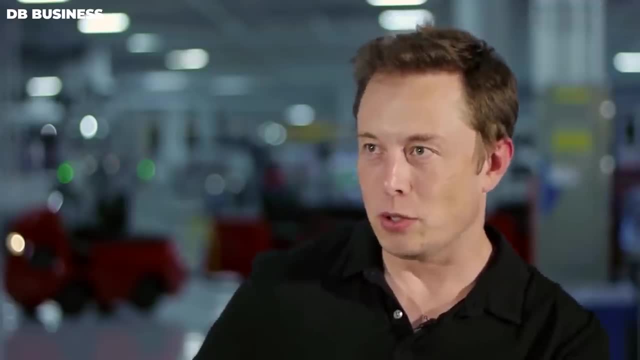 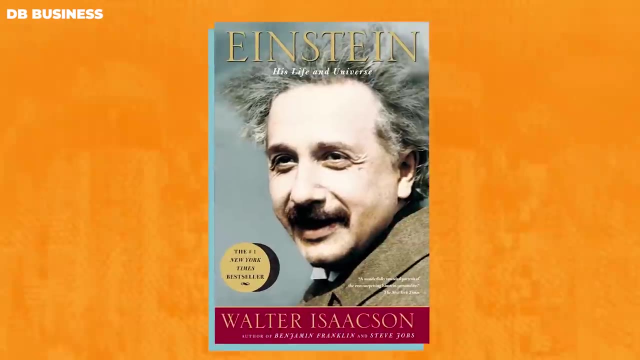 It also comes as no surprise that Musk recommends books about other geniuses who have lived, notably the book Benjamin Franklin, An American Life by Walter Isaacson, As well as Einstein, His Life and Universe, also by Isaacson. From reading all those books, 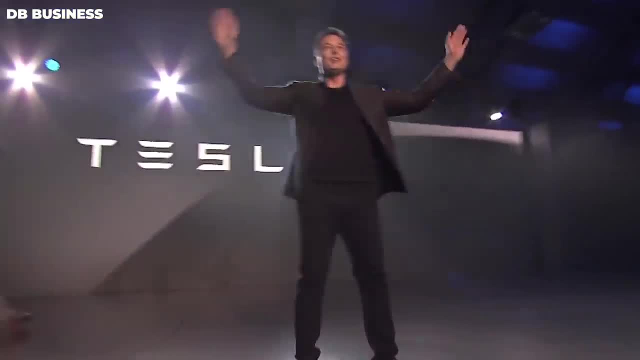 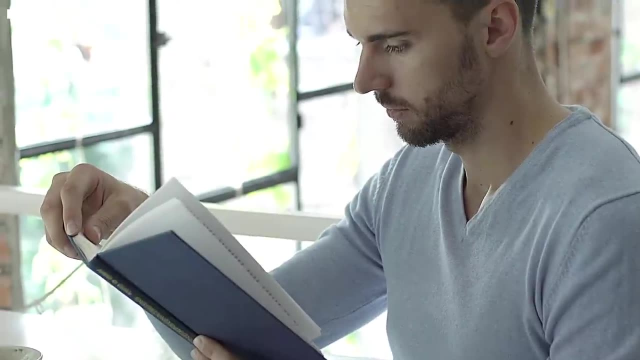 Musk learned a great deal about leadership and purpose to change the world for better place. Although the average person probably doesn't have 10 hours a day to dedicate to reading, some of the richest and most talented people will tell you that one of the secrets to their success. 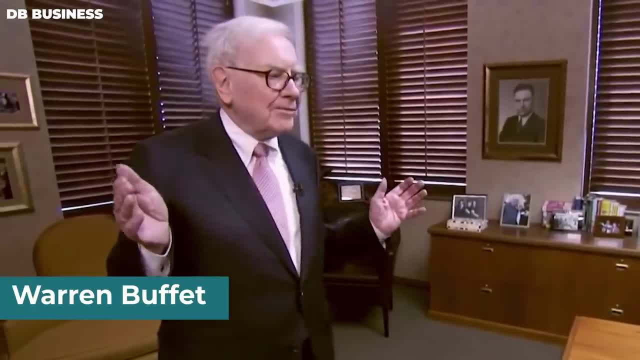 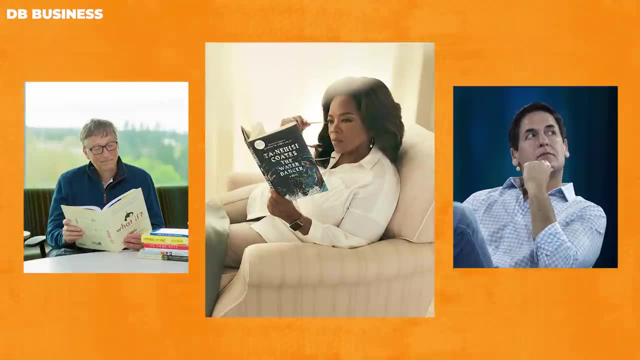 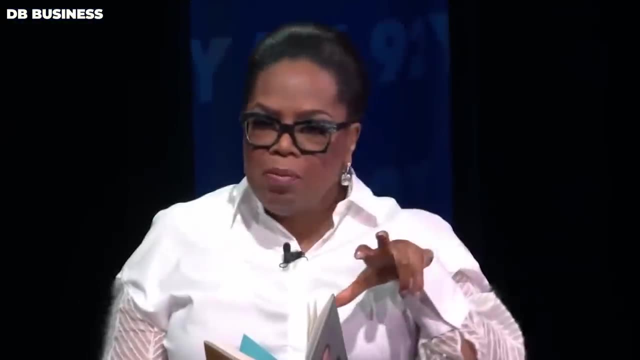 is that they read constantly. Warren Buffett reportedly reads between five to six hours daily, making his way through a handful of newspapers and financial documents. Other billionaires such as Bill Gates, Oprah Winfrey and Mark Cuban all attest to the power of reading and the impact it has had on their success and business acumen. If you are interested, 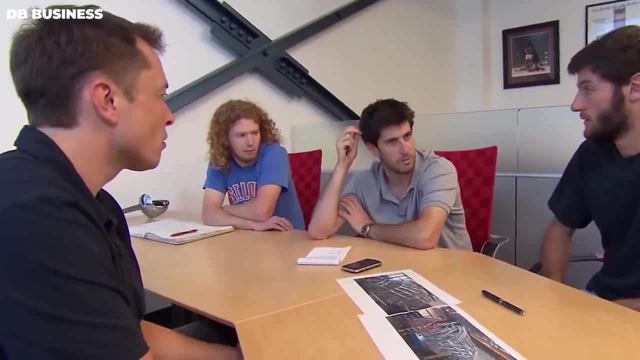 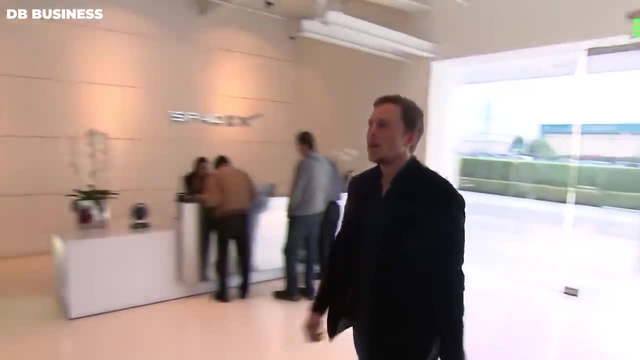 in building your knowledge through books the way Musk has done it won't guarantee that you will be on the level of a rocket scientist in a short amount of time. Musk can't even call himself a proper rocket scientist. He simply accrued an impressive amount of information, But what?